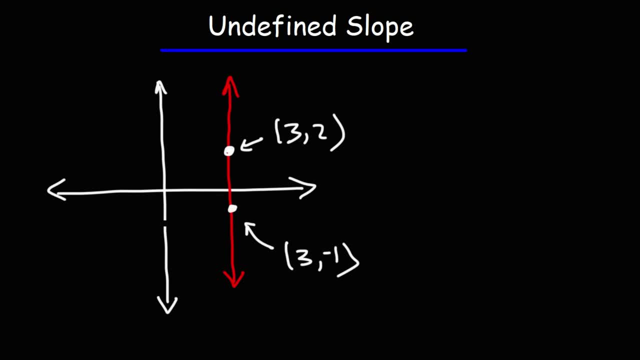 Calculate the slope of the line using those two points. To find the slope we could use this formula: It's rise over run. It's y2 minus y1 over x2 minus x1. So we could say this is x1, y1, and we could define this as x2 and y2.. 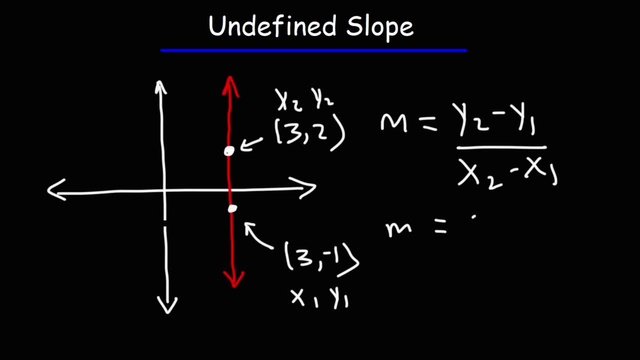 So using that formula, we have: y2 is 2,, y1 is negative 1,, x2 is 3, and x1 is 3.. 2 minus negative 1, that's the same as 2 plus 1, which is 3.. 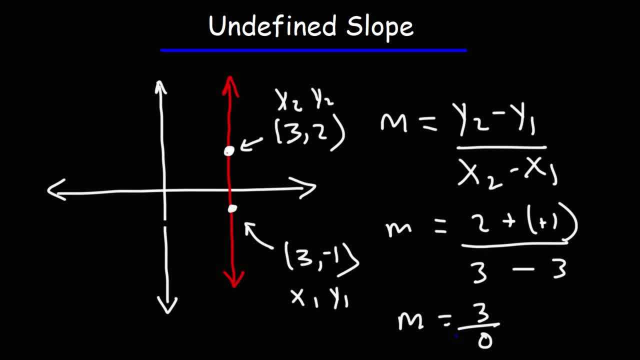 3 minus 3 is 0.. So notice that we have a 0 in the denominator of the fraction. So that tells us that this slope has an undefined value. Anytime you have a vertical line, the slope is always going to be undefined. 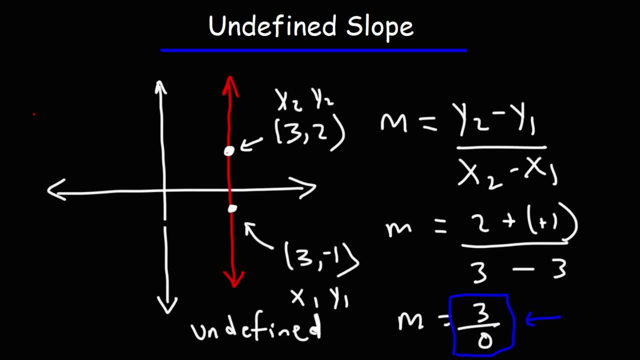 Now let's compare that to a horizontal line. Let's say we have a line right here And let's identify two points on this line. Let's say this point is at negative 5, comma 3.. And we'll say this point is negative 2.. 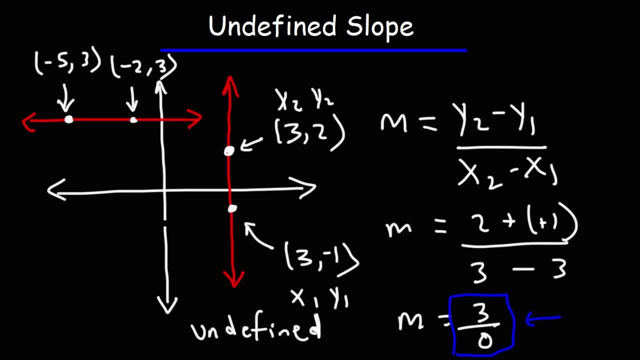 Let's calculate the slope of that line. Let's see why it's going to be 0.. So this is x1, y1,, this is x2, and y2.. So, using the same formula, y2 is 3, y1 is 3, x2 is negative, 2 minus x1, which is negative 5.. 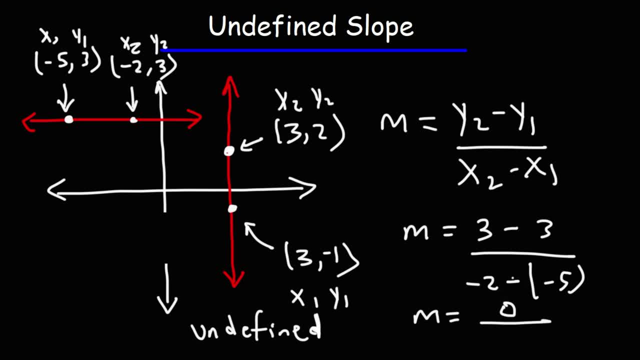 3 minus 3 is 0.. Here we have negative 2.. Negative 2 plus 5,, which is positive 3. So anytime you have a 0 in the numerator of a fraction, the entire value of that fraction will be 0.. 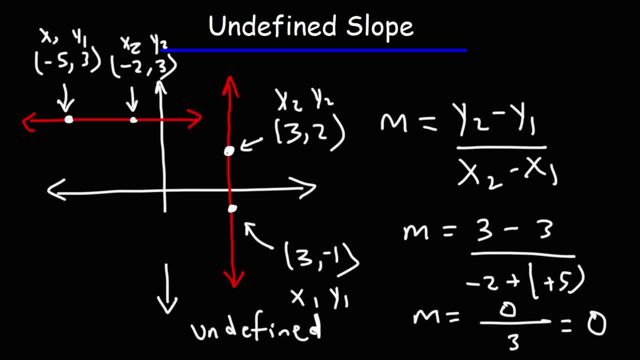 So it doesn't really matter what the x values are. The slope of a horizontal line will always be 0. And the slope of a vertical line will always be undefined. Now, what are the equations Of these two lines? How would you describe their equations?